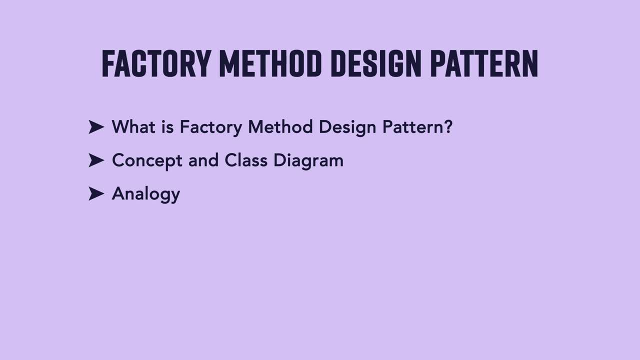 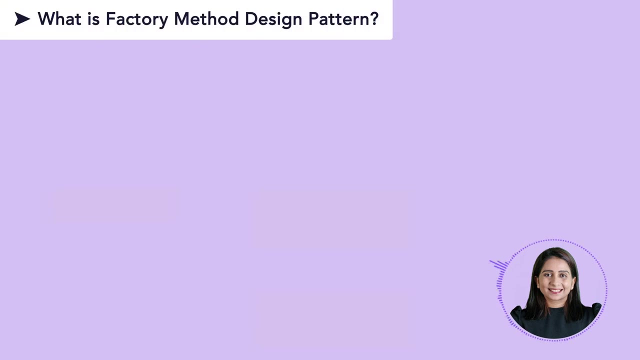 analogy to. where does the thinking of factory method design pattern comes from? Then we will have a short code walkthrough and in the end we will summarize with pros and cons and summary for this video. Let's first understand what factory method design pattern is Starting from the 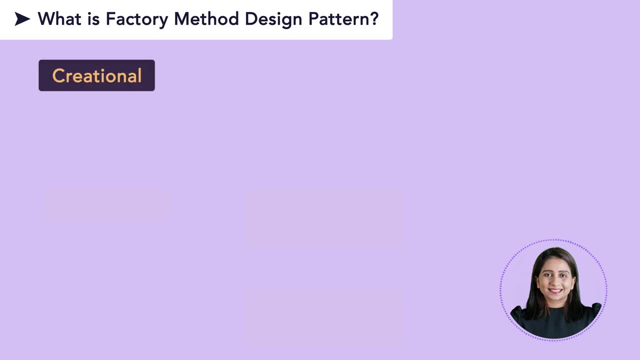 fundamentals. it is a creational design pattern. It is used in order to create objects of classes or to instantiate objects. The catch, however, is that it is used to create the objects which can be of similar type, or which are usually of similar type but vary a little in terms of implementation. 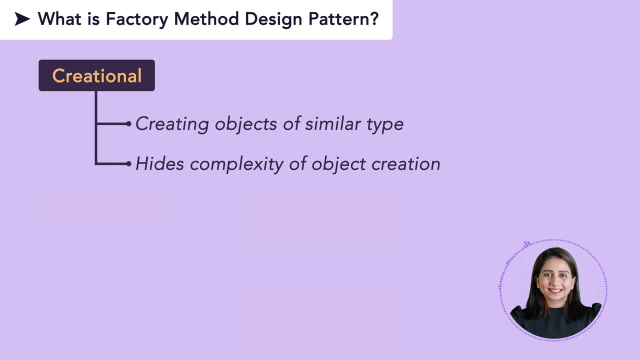 The goal of factory method pattern is to hide that complexity while creating such objects which are of similar type but can have different implementations. So the client code, which is actually using the factory method pattern, has no idea how those objects are created. Let's try to understand this using a box diagram. Let's say that this is your client code. Client. 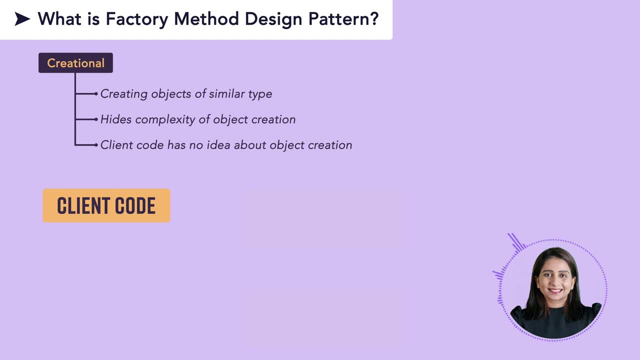 code could be any other application calling your code or any other module application calling your code, which calls an interface or a function which resides under a factory method interface. Now this client code will just call that function which is exposed by this factory method interface. Let's call that function as f1 or any other function for that. 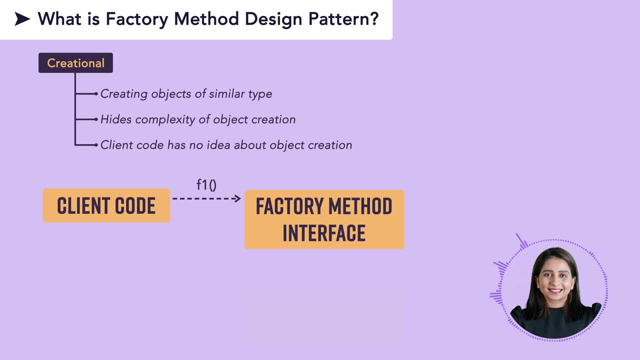 matter Now. this f1 function is going to return the instance or the object that client code is expecting. However, the beauty here is that this interface does not expose to the client what is the complexity in creating that object, because this interface does not implement how that object is created. That implementation is deferred or is. 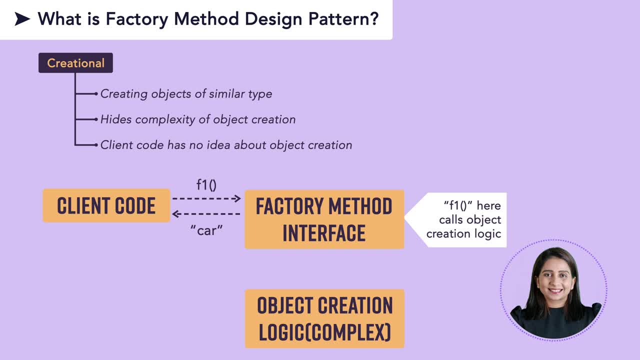 left up to the classes which are implementing the actual logic to initialize those objects. So you can see this particular box here where that instantiation is done. In terms of classes, this particular box or this particular code here is also called concrete classes or subclasses, which actually implement the code in order to initialize. 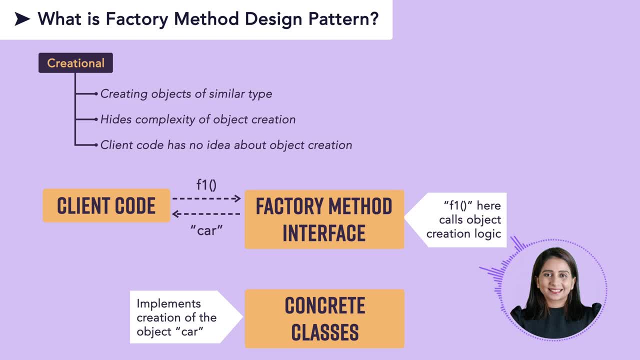 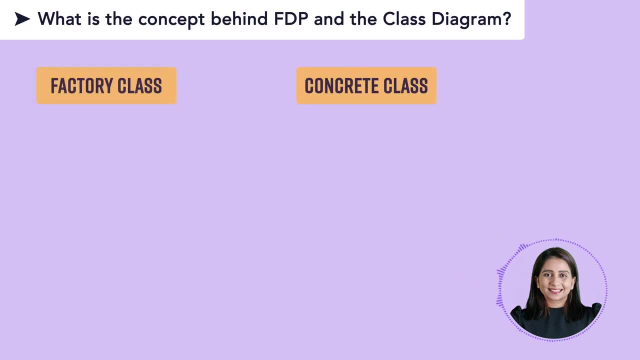 objects, which is hidden behind this factory method interface. Let's move on to see the class diagram. If we see the class diagram right here, you can see that there is this factory class which will be the abstract interface. It will have a method as factory method. It is a convention used while 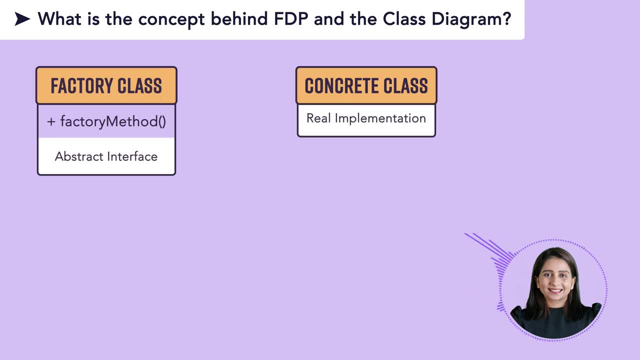 implementing factory method pattern. and then there will be a concrete class which will be a subclass class of factory class or it will be inheriting from factory class. it will be implementing the function which is defined in this interface here, and this is the function which the concrete 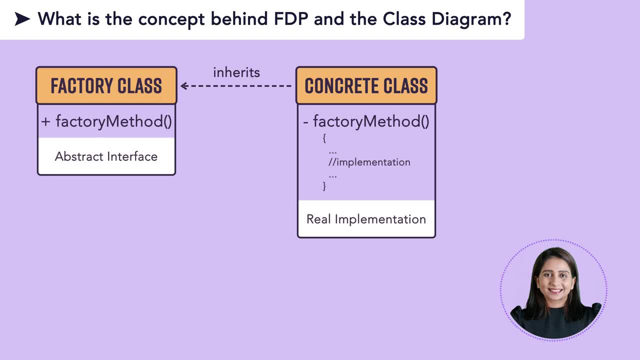 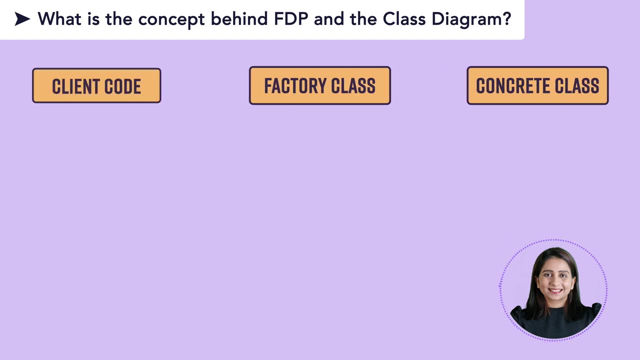 class actually going to implement. So, as I said, this particular class is the abstract interface and this particular class is the actual implementation. Let's try to understand this class diagram using an example, as we just discussed, that client code is going to call a function like create vehicle with some parameters heavy. 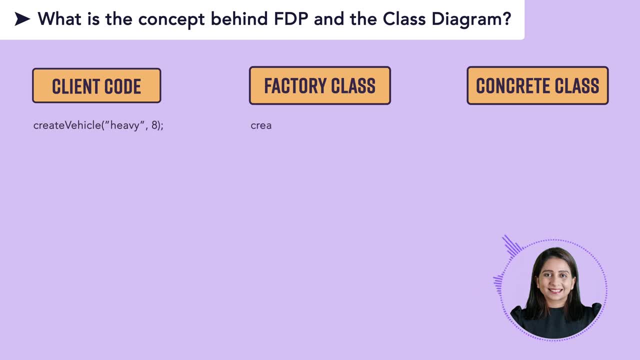 and number of wheels as 8.. Now to the client. this is the only function which will be exposed to Now in the factory method class itself, this function will not be implemented. only this interface will be shown or this signature of this implementation will be defined in. 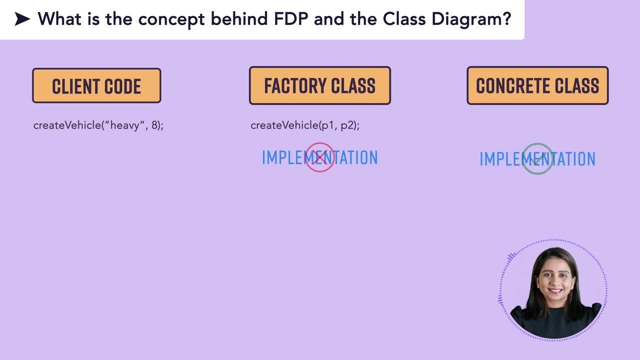 the factory method class. However, the real implementation will go to the class which implements this interface. Now, this particular method in the concrete class- create vehicle, P1, P2- will check if P1- P2.. P1 is equal, equal to heavy, and, and if P2 is equal- equal to 8, then create truck. if these 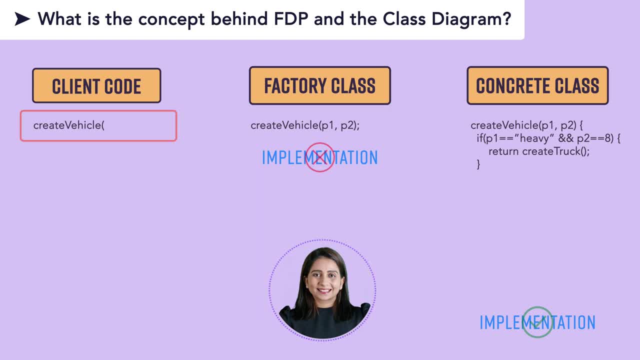 parameters would have been something else, such as light and 4. instead of creating truck, it will be, as we can see here. it will be P1 equal- equal to light and and P2 equal- equal to 4. it will be create a car. This is a very, very simple example of how the implementation would be done, but the important 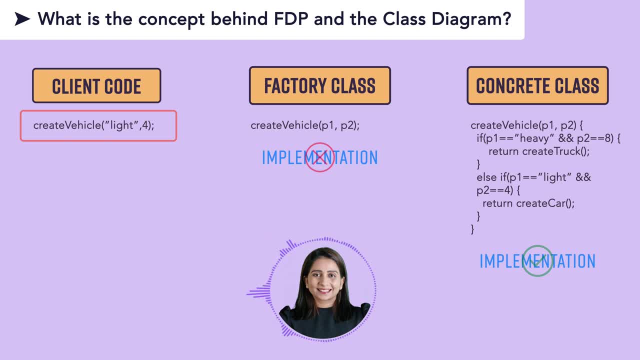 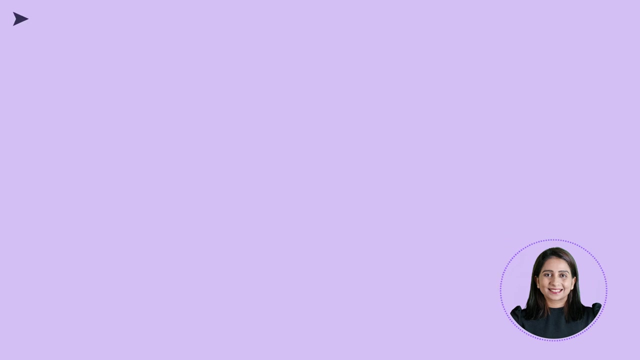 point to note here is- which you must have guessed by now- that this particular implementation is hidden from this interface and the client, who is actually calling this function, has no idea about this implementation. This is how factory pattern hides complexity. As you all know, I like to use analogies to explain difficult concepts, so that they can 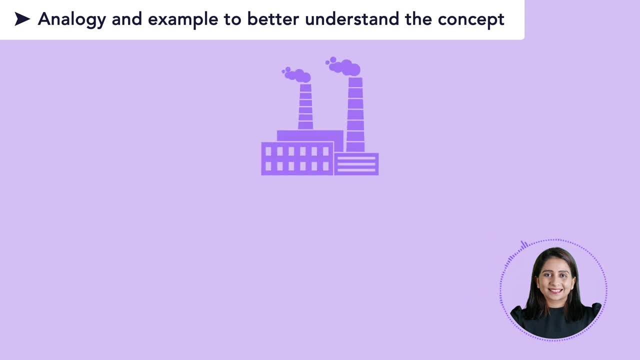 seem very simple to us. Let's take example of a factory. This factory creates bottle lids or it manufactures bottle lids. It does not manufacture the actual bottles, but it manufactures the lids that are used on bottles. Since it's a factory, it is producing different types of lids. 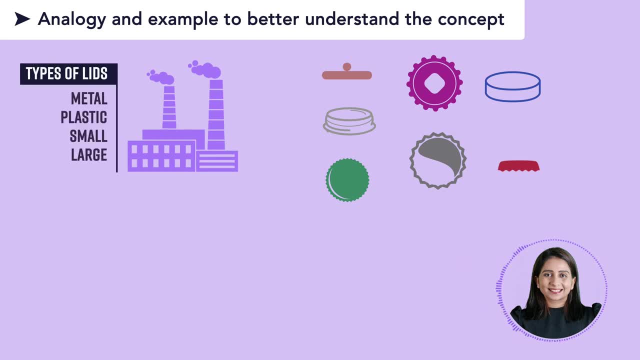 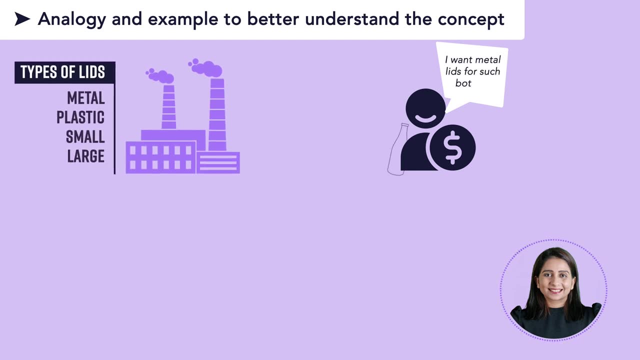 It can be metal lids plus plastic lids, small or large lids, and so on. now the client who is coming to place an order, The factory would just say that I want lids made up of metal for certain kind of bottles. The factory might have different departments and different divisions to create different. 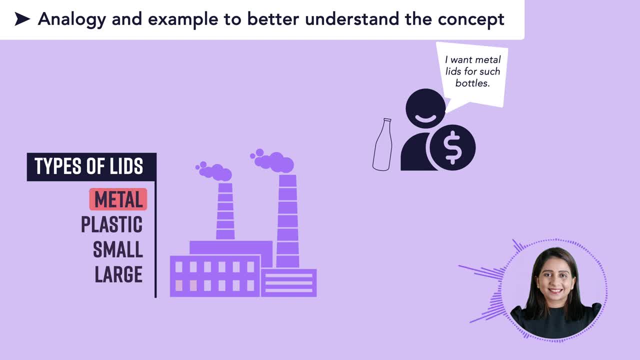 types of lids and it would be creating metal lids somewhere else and plastic lids somewhere else, and they might even have different machinery to do that. but client has no idea about that. Client just says: create lids for metal and might give number of lids like 6400 and so 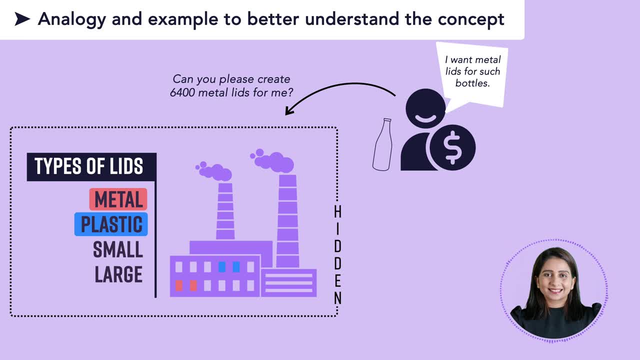 on. It's just a random number that I'm using. The factory itself hides how it does it, but it returns those 6400 lids to the client that has requested or placed this order. This is the exact same concept, which is applied in code, while we are creating objects, which 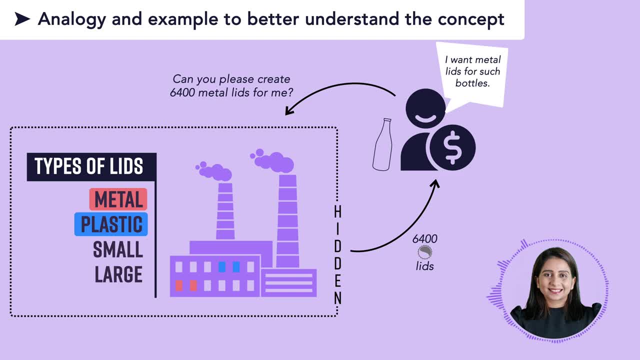 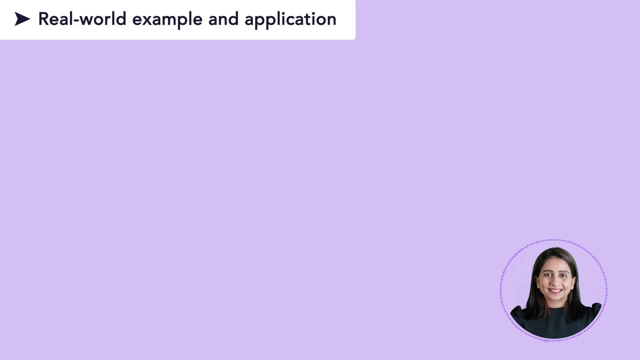 are complex to create and which might depend on some parameters which we receive from client. We do not expose all that complexity to the client. Now one may argue: what would be the real world application of this factory method design pattern, or where would it be used? 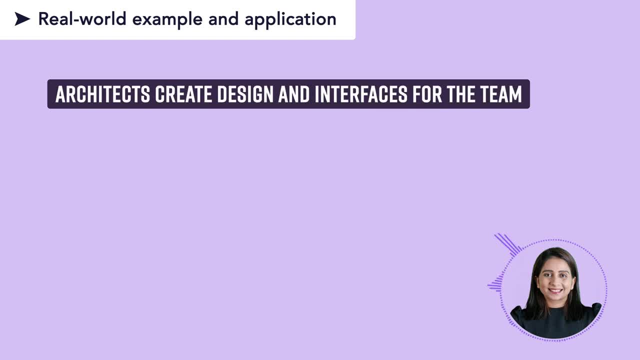 It is a very common design pattern utilized when architects want to create the code base and there are different developers who are going to implement those interfaces or implement that code base when creating certain objects which are complex and which cannot be created just by using one class. 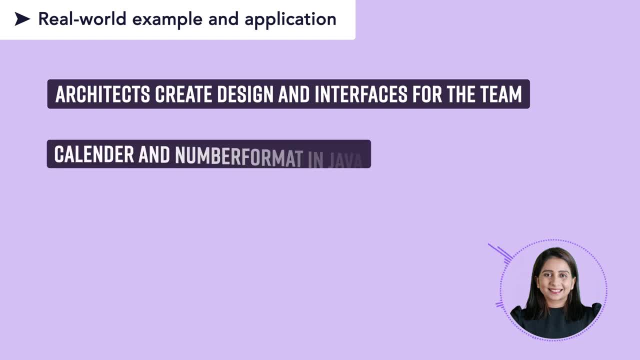 That is one application. Another application is that you can actually go and check out the calendar and number format classes in Java. Those are the classic examples of how factory method design pattern is implemented. Another example, Another application of this pattern is while somebody is developing frameworks in library. 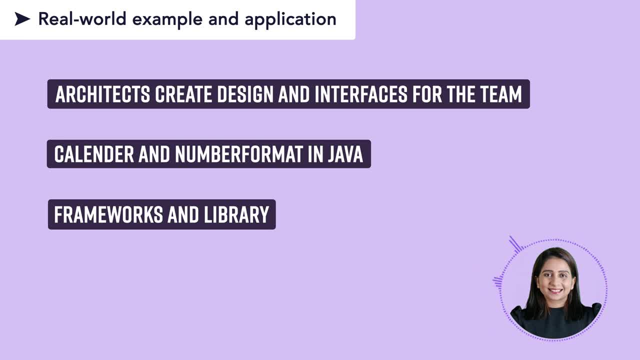 You might have come across where you yourself would have used a library, but the people who are implementing that library. let's say that someone is implementing a UI framework and they want to give you the option to create different types of buttons, scroll bars and widgets. 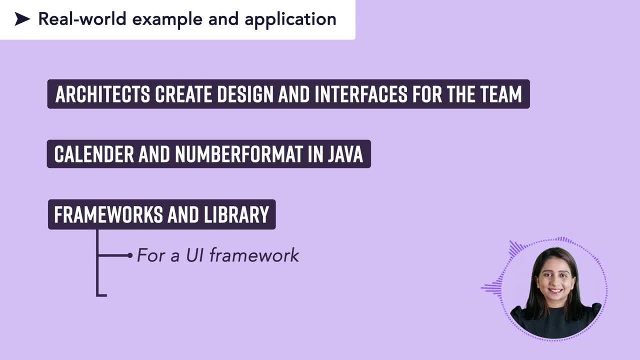 They might be using the factory method design pattern so that you can initialize different kind of buttons depending on your parameters. Note that You don't get to see how that code is implemented when you're using that library, But when you dig deep into the source code you can find out that they might have utilized. 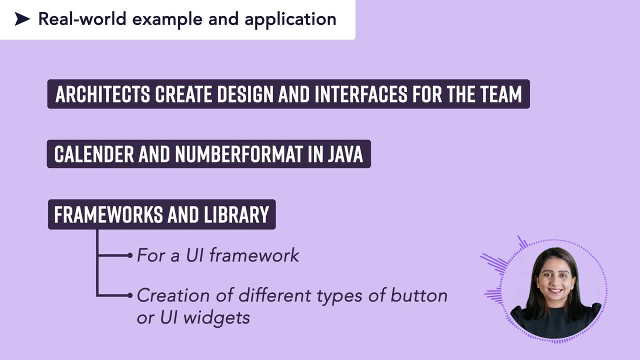 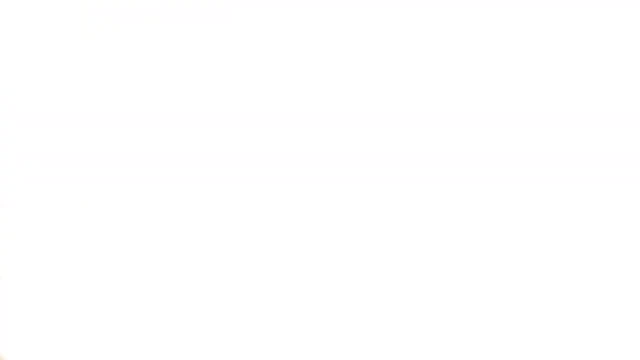 the factory method design pattern in order for you to create those objects. So this is about the real world application of factory method design pattern. Now we will move on to the code walkthrough, but before I start showing you the class diagrams and the actual code, I just want to give you a brief idea what problem or what we are building. 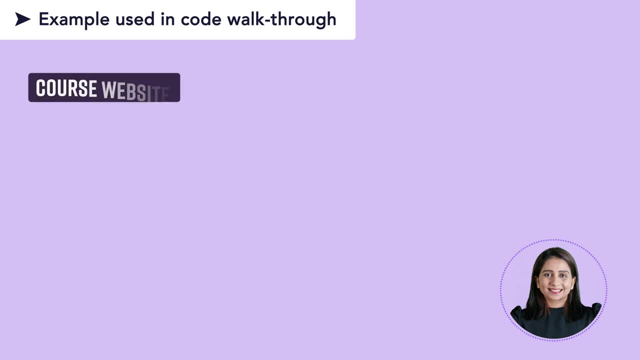 using this example. So let's say you have to build a course website, just like edX or Udacity etc. where that website has multiple online courses and every course can have same or different kind of modules. So there is one website, It will have multiple courses and every course will have different modules. although I have 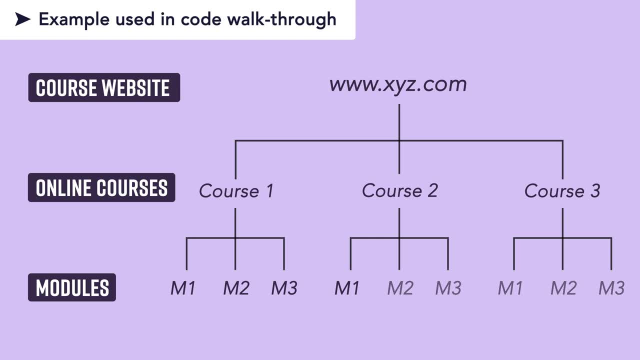 written here: M1,, M2,, M3 for all of them, but it can be something else as well. So just to give you an idea, That One course can have common modules with others, but it can so happen that one course has no. 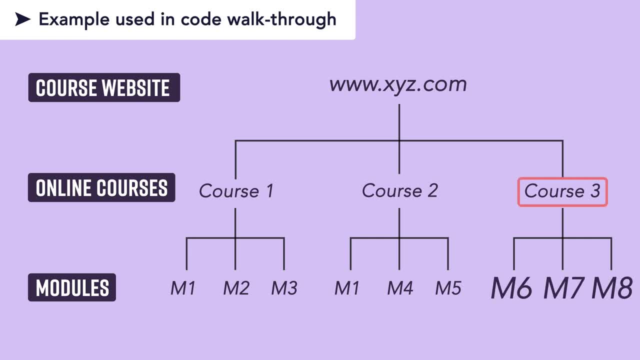 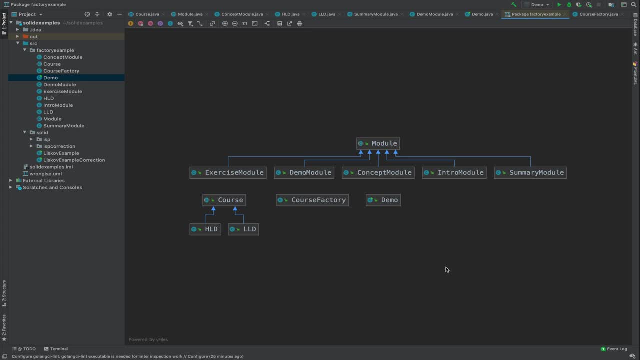 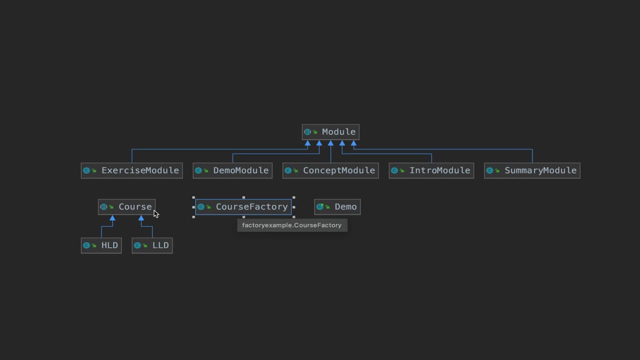 common modules with others. Now we will jump to the code and see how all of this is done using factory method design pattern. Let's start the code walkthrough with the class diagram. As you can see here that we have the course factory class. This is going to be the factory class that we refer to in the diagram we saw before. 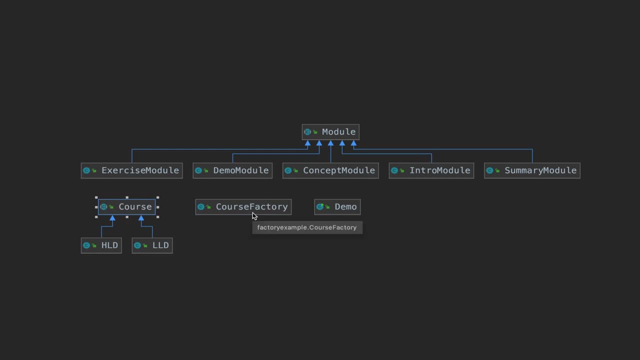 This is the course class, which will be the concrete class implementing the interface defined in course factory class, And then HLD and LLD are just the subclasses which have inherited from course class. The demo class that you see over here is actually the client code or the client class that we 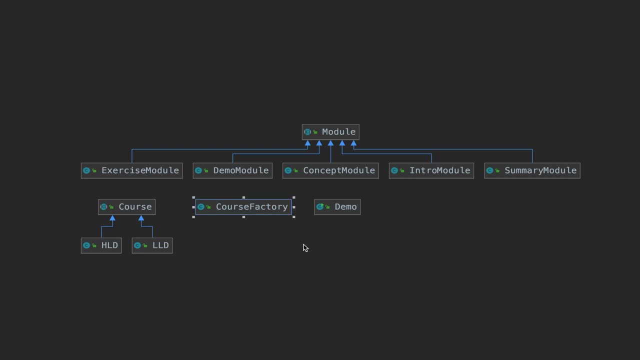 have seen in the example, who has no idea how course factory is returning the objects of course to the demo class, where the actual implementation is hidden behind this course class and the HLD and LLD classes. The module classes over here are nothing but just the modules that a course is composed. 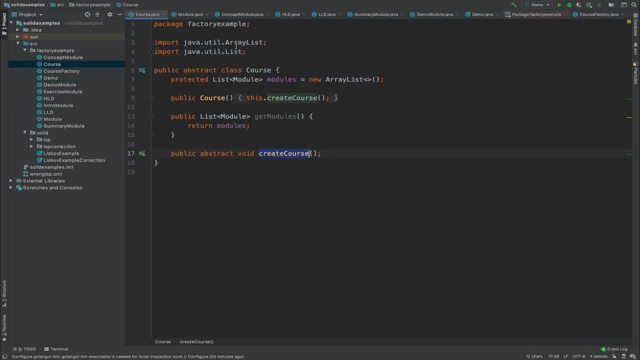 of. Let's start with the course class first. So, as I said that the course has multiple modules, If you just go and check what a module class is, you can just see that I have just created an abstract class and then there are multiple modules which extend this particular module. 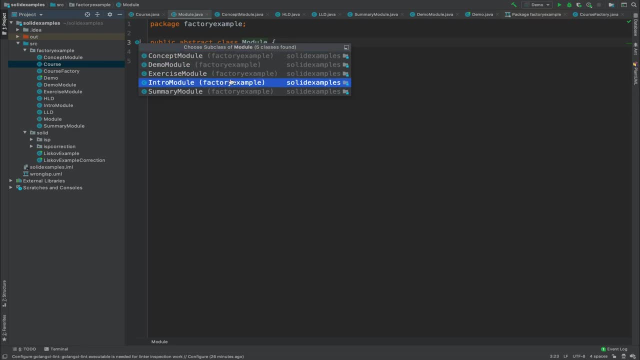 class here and every course can use one or multiple of these modules. Coming back to course class, there is this constructor here and a simple getter for get all the modules. Now, the important part of a factory method design pattern is this particular line of code where we have declared an abstract function of create course which will be implemented. 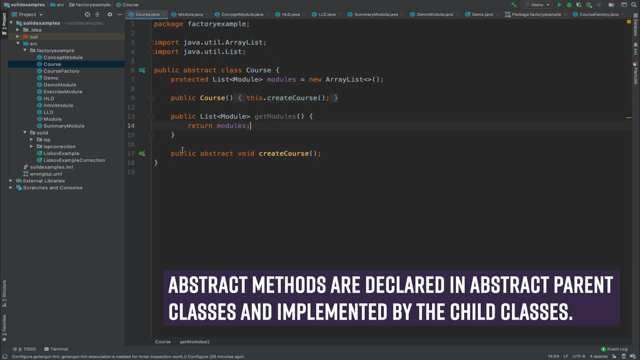 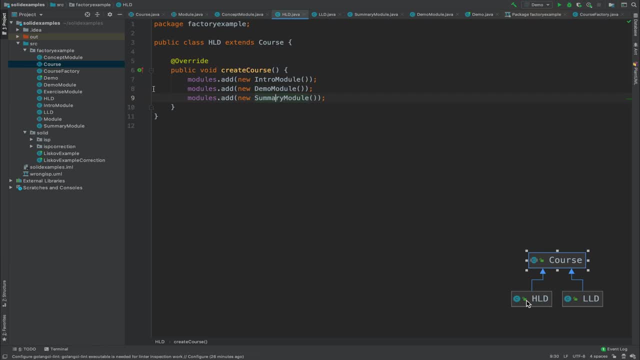 by the classes which are inheriting from course class here. So this particular method is implemented by HLD, where it has the modules which are utilized in the HLD course. Similarly it is also implemented by LLD class, where it has modules which are specific to. 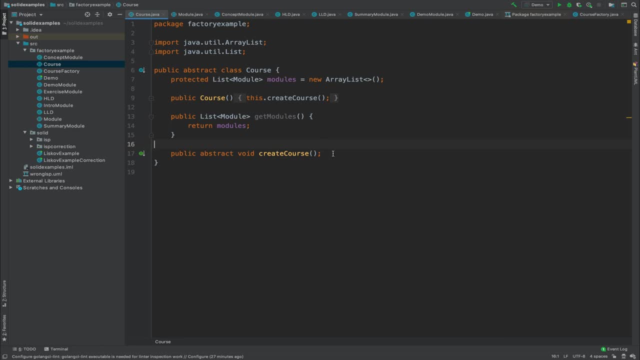 LLD classes, As you can see that every class has its own implementation. So if somebody wants an LLD course, the specifics of LLD course are not same as specifics of HLD course. So if someone wants an LLD course object, they would have to use the LLD class. and if 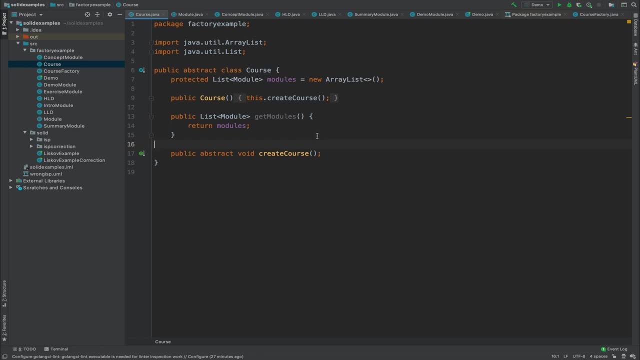 someone wants an HLD object, they would have to use the HLD class. Now, who is handling this particular code? This particular code is handled by the course factory class. It checks from the caller. If the course type is LLD, return the object of LLD. 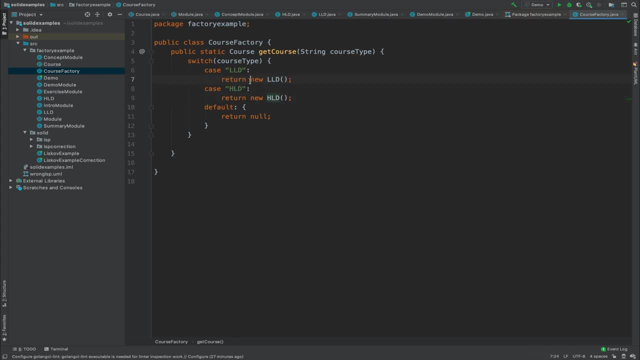 If it is HLD, return the object of HLD and the actual implementation, as you can see, is hidden in this LLD and HLD classes. Now, who calls this particular get course function? It's our demo class, which is the client code. 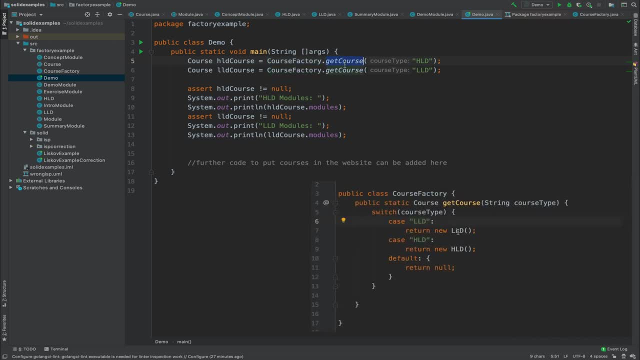 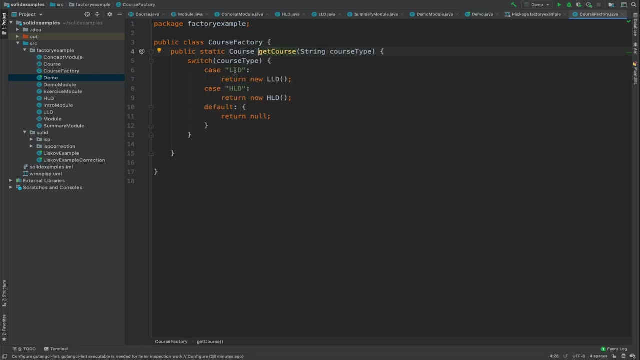 The client code only depends on the course factory in order to get the object of a particular course, either HLD or LLD, and this function get course in the course factory, depending on this parameter. Either calls LLD or HLD. So all the magic lies here in this particular switch case, as well as in this course class. 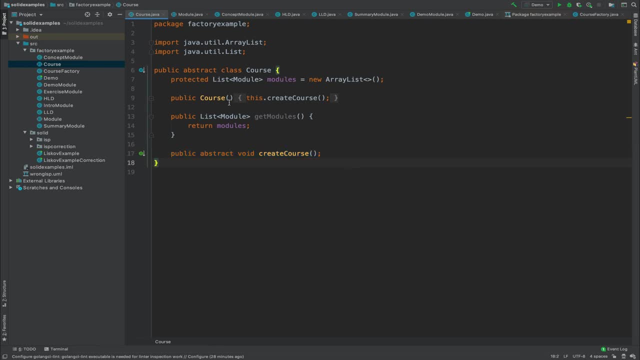 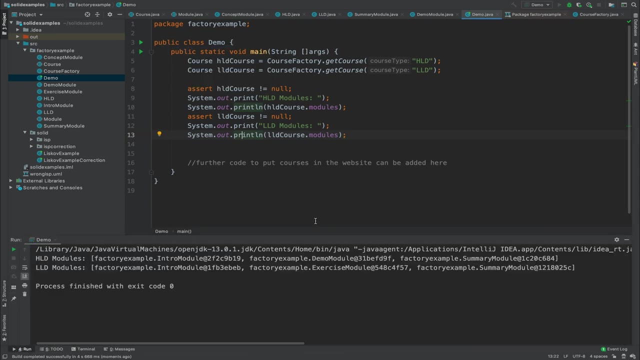 where we have declared this particular function create course as abstract. Now let's see how this particular code runs. So, as you can see, here the HLD modules are different from the LLD modules and this is how factory method design pattern is implemented. 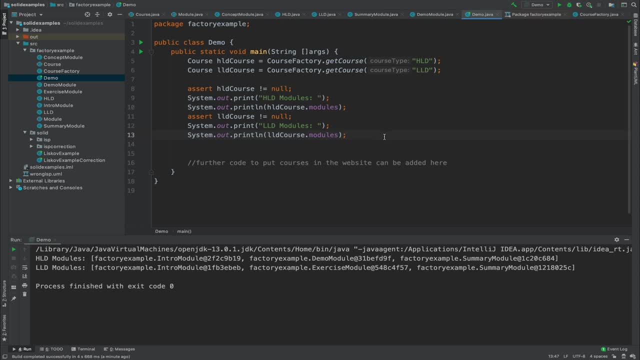 So this was a brief code walkthrough, Thank you. If you have any doubts regarding the same, please feel free to leave them in the comments. So that was a brief introduction to the basics and fundamentals of factory method design pattern. If you understand this pattern properly, it will be very easy for you to build your understanding. 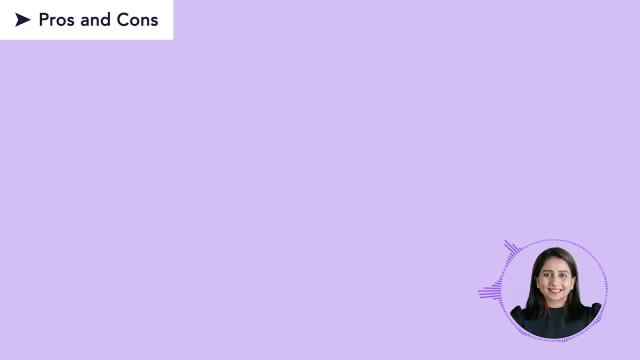 for other patterns. But having said that, let's also look at the pros and cons of this factory method design pattern. Now, as you can see that the pros are that this pattern is very easy to understand, and it is very easy to understand. 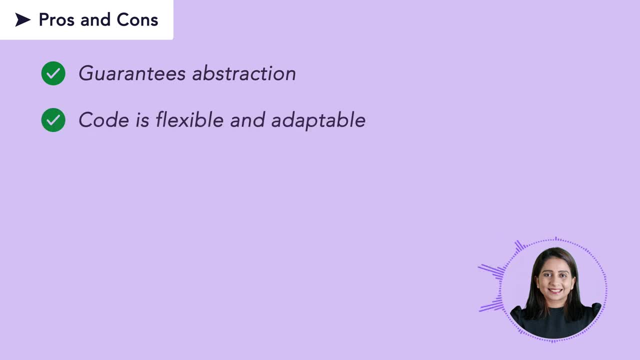 So let's look at the pros and cons of this factory method design pattern. The pros are that the design pattern guarantees abstraction and the code becomes flexible and adaptable. If you want to add different types of object creation to your code, you can do that. 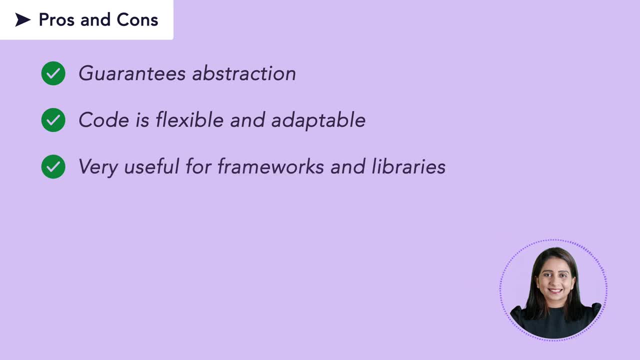 Also factory method. design pattern is very useful for implementation of frameworks and libraries. Now, since we are learning about design, whether it is low level design or high level design, every kind of design pattern or design has some upsides and downsides. 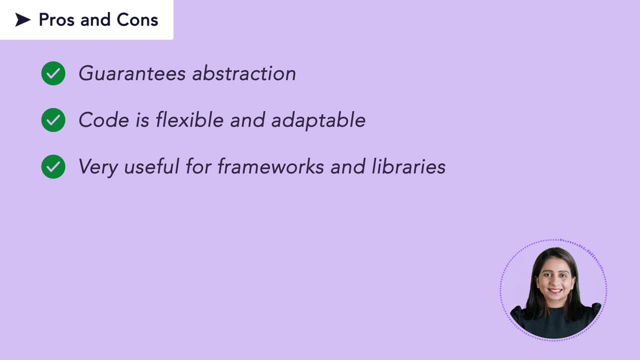 And there are some downsides to factory method design pattern as well. First one is, as you might have already seen, that the code becomes quite complex And it becomes a little complex to demo or understand as well, And it takes time to set the base in order to write the factory method design pattern. 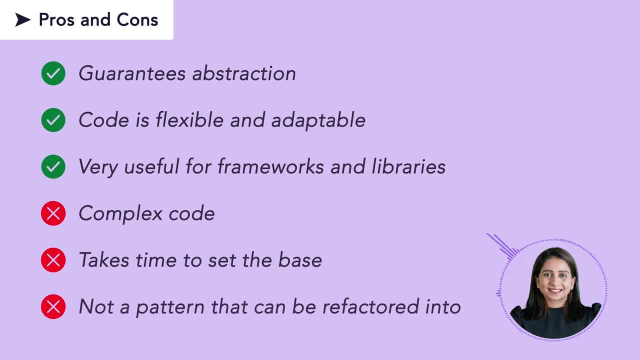 or implement it. Also, it is not possible for you to refactor your code into factory method design pattern, meaning you would have to start from scratch to write or implement factory method design pattern if you're going to create objects that are complicated to create. 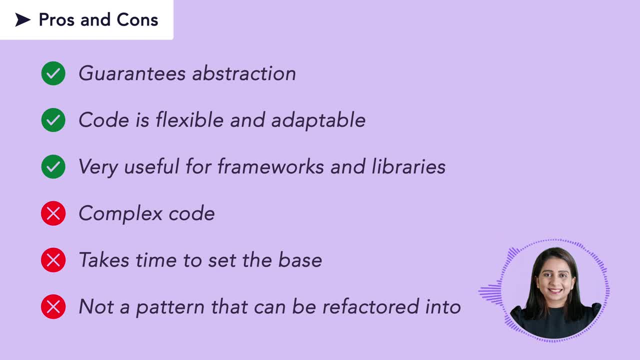 It's not like that. first you write different classes to create your objects and then you try to refactor it into factory method design pattern. It's not like that. And it's not like that. if you're complimenting the design, You are actually continuing to listen to the design co-creator and then try to refactor.